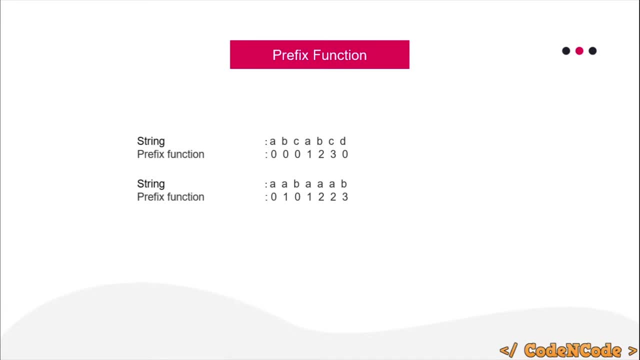 depends upon prefix function for its implementation. So prefix function, the definition. we have already seen. this is an example of prefix function. So here you see, for i is equal to 0, I will be considering 0 base index system. So character a is at index 0, this is at index 1, and so on. 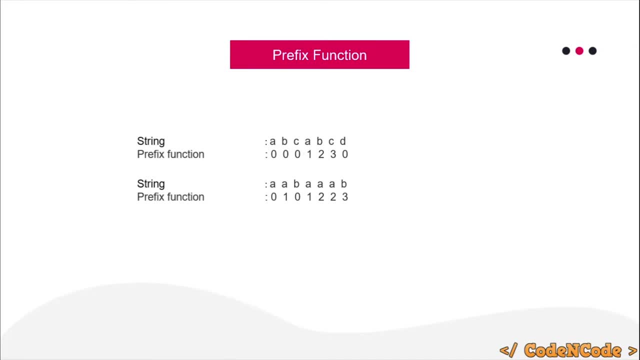 So we are using here the same index system which strings use. So we will be using 0 base index system. So pi of 0 would be 0, because it has no proper prefix. Pi of 1, it has one proper prefix, that is a. 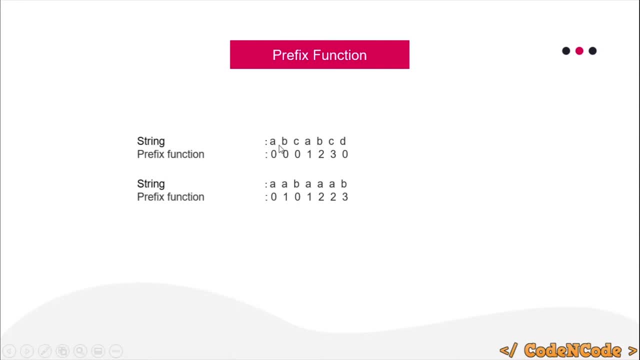 Right, So the whole substring is ab and the proper prefix is a, So proper prefix a is not equal to proper suffix of length 1.. Length 1- proper prefix is only a and length 1 proper suffix is only b. a is not equal to b, clearly, so the answer is 0.. 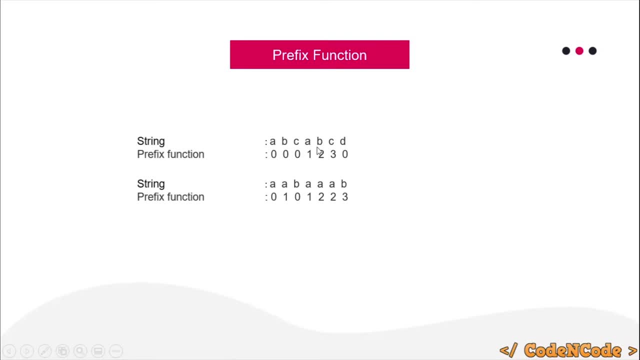 Similarly for a. for this abca string, if we see proper suffix a is equal to proper prefix a And that is why the length, the maximum length, suffix a is 0. So the answer is 0.. The length suffix, which is also equal to prefix, is 1. that is why pi of 3 is 1. similarly for: 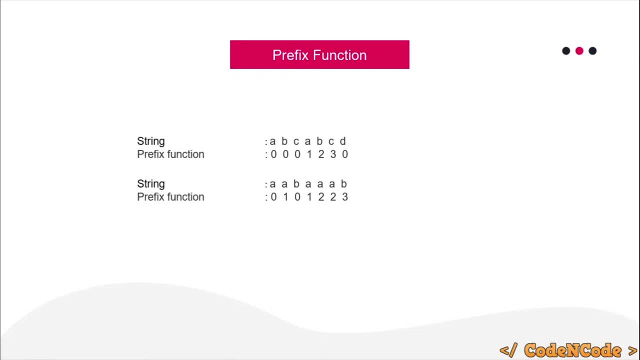 the rest of it. You can read more about them on the cpalgorithmcom the link I will be posting in the description of the video about the prefix function, because I already told you this whole course. I am following cpalgorithmcom as a reference, so I will be providing the link in the description. 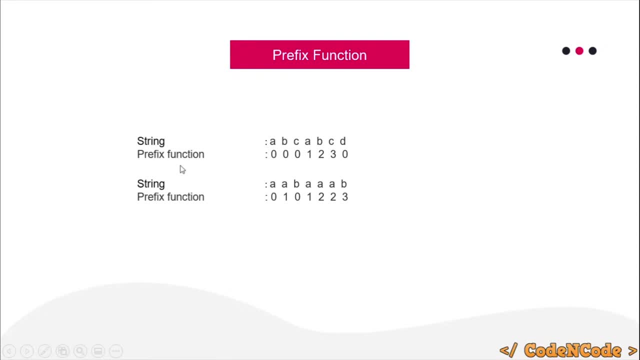 so you can learn more about this. For example, here you can see the prefix aa matches. sorry, the suffix aa matches prefix aa and that is why the prefix function, the value of pi function at this index is 2.. For this, aab matches the prefix, the suffix aab matches the suffix prefix aab, that is. 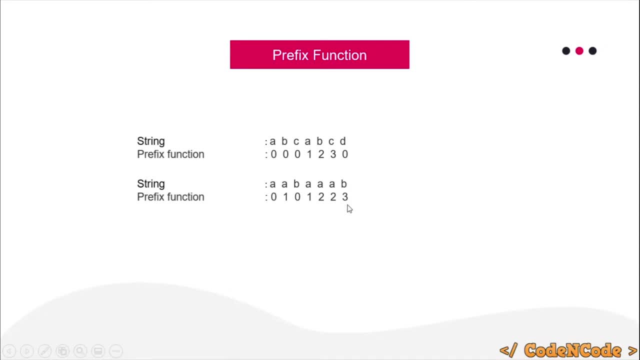 why pi of this index is equal to 3.. So the question is how you can compare. It is easy, It is very easy. For example, if you are going to calculate for substring 0 through this, so 0 through 6, what you can do you can first compare length 5 prefix and suffix. length 5 prefix is a through. 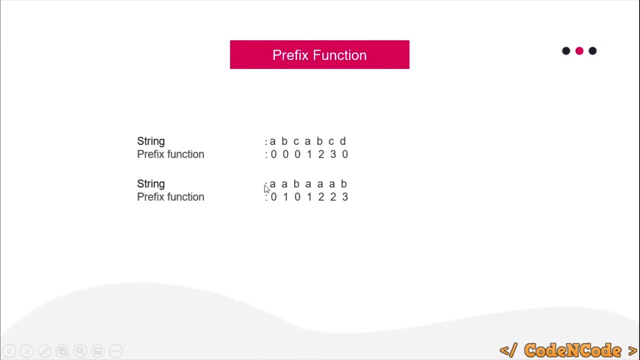 this, I guess. ok, 6, so you can start the whole string. I am talking about the substring 0 through 6, right, sorry, 7 characters. Indices are from 0 to 6.. If you want to calculate pi of 6, then you would. since there are 7 characters, you would start. 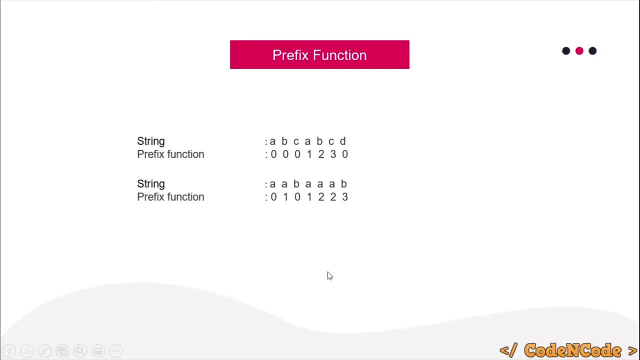 with 6 character prefix. So 6 character prefix would be aa, b, aaa, and you will be checking whether this 6 character prefix is equal to 6 character suffix or not. So we see 6 character suffix is ab or aaa b, which is not equal to 6 character prefix. 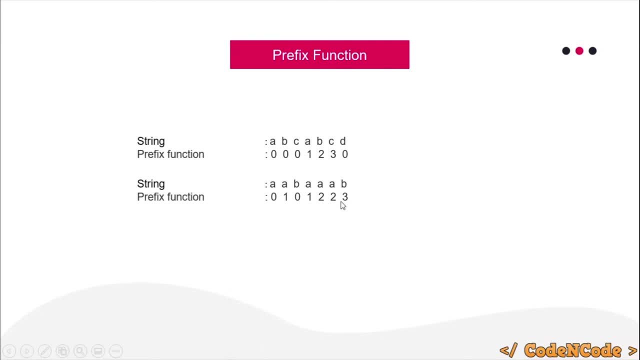 So 6 is not the answer, Then you will be going for 5. And then you will be checking for 4, and then you will be checking for 3.. So 3 character prefix is aa b and 3 character suffix is aa b as well. 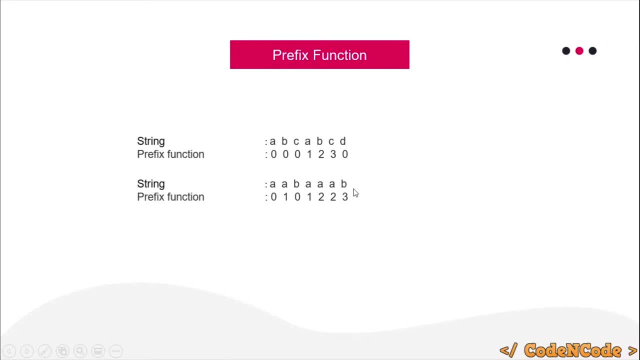 So you can see, 3 character prefix is equal to 3 character suffix, and that is why the answer is 3, which is the maximum you can achieve. So that is why the prefix or the pi of index 6 is equal to 3.. 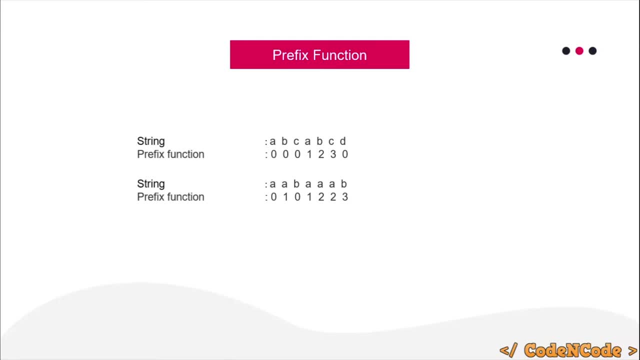 So that is why the prefix or the pi of index 6 is equal to 3.. Now the naive approach. The first one is the index 6.. You can use the naive approach to calculate this, and if I show you here, This is the code. 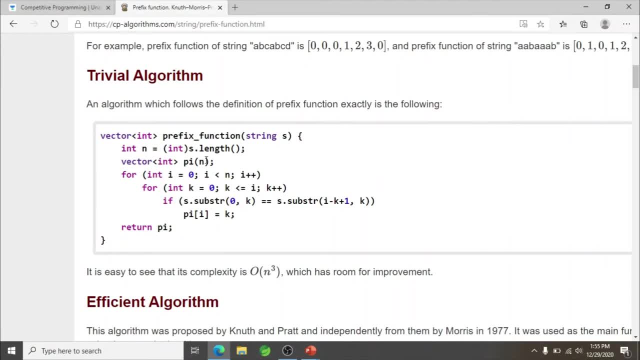 Let me increase the font size On the cpalgorithmcom, the link I will be providing in the description. So this is the naive approach you can apply where we are running two nested for loop and checking the substring. The overall complexity is n-cube. 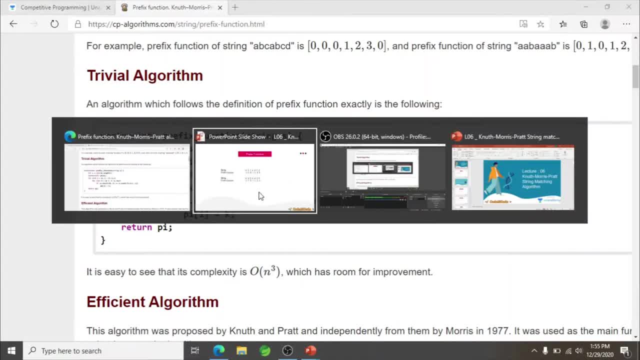 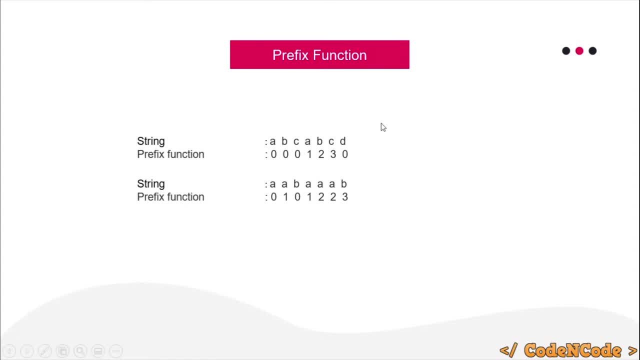 You can read about it. This is very, very basic so I am not going to explain this. You go there and try to understand that algorithm. That is very, very easy. The thing that I have explained here that go for 5 character prefix and suffix, then go. 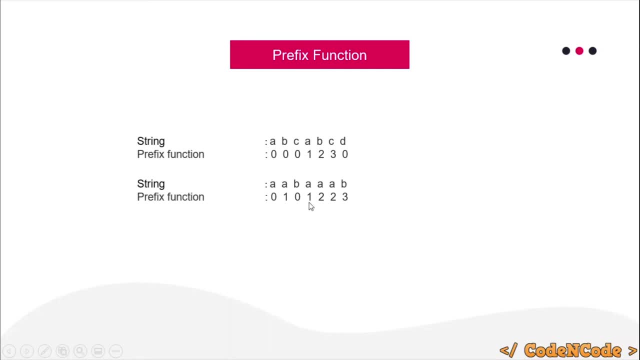 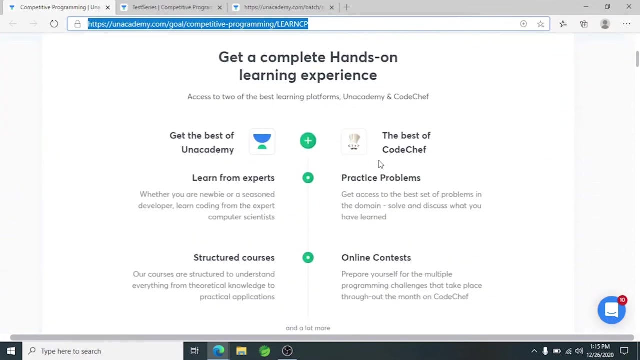 for 4 character, prefix and suffix. That is exactly what is happening there. Understand that first before moving on, because understanding of how prefix function actually is calculated is very, very important. Speaking of algorithm, one of the best learning platform Unacademy and one of the best practicing- 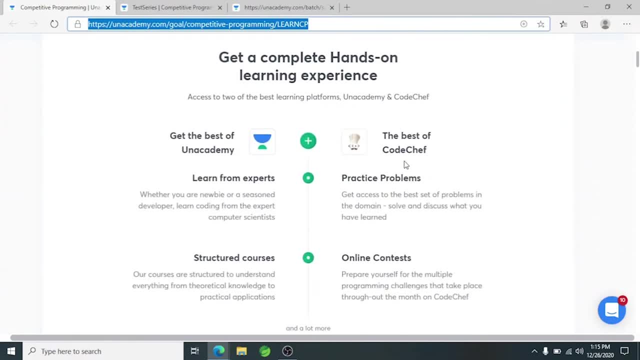 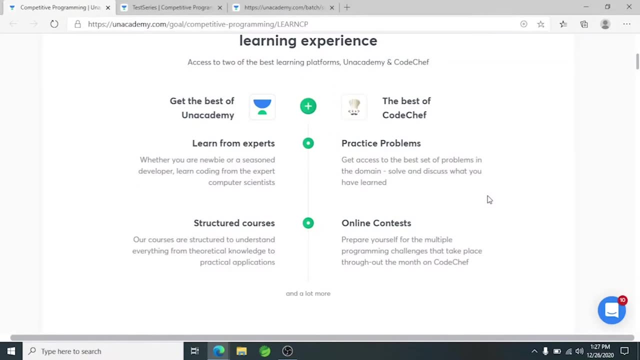 platform, Codechef, are coming together to help you get better at programming and problem-solving. Unacademy knows how important it is for you to monitor your progress throughout the course, so they have provided a series of mooc tests which will help you monitor your progress. 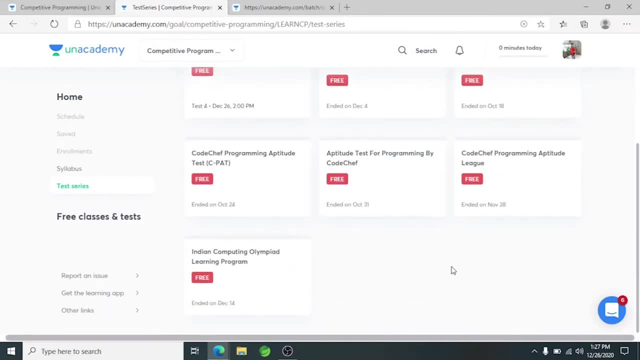 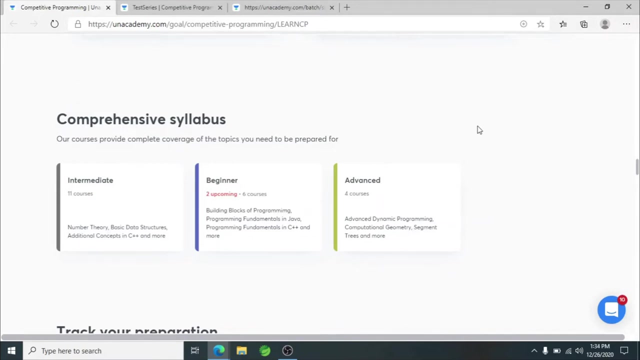 throughout the course, which you can take and which will also help you analyze the area which require improvement. These courses provide right kind of guidance and structured learning for every level of programmer, whether you are a beginner programmer who has just started with competitive programming, or an intermediate programmer. 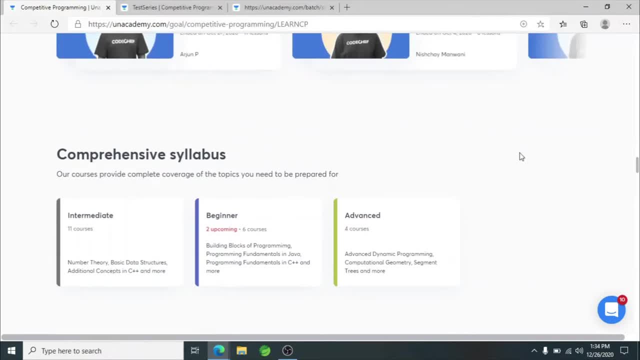 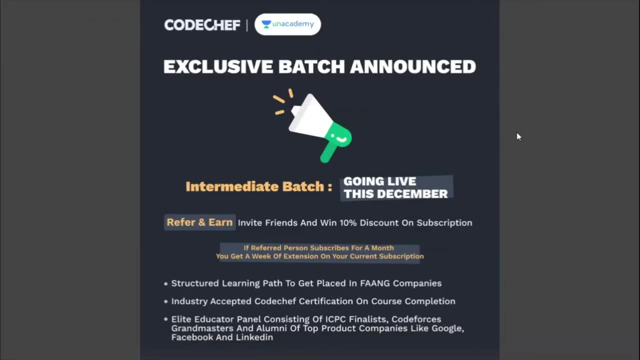 An academy has summit batch, which can help you improve your chances of getting placed in fun companies. It can also help you crack international coding competitions like ACM, ICPC. Not only that, if you go for 6 or 12 months subscription, you are eligible for industry. 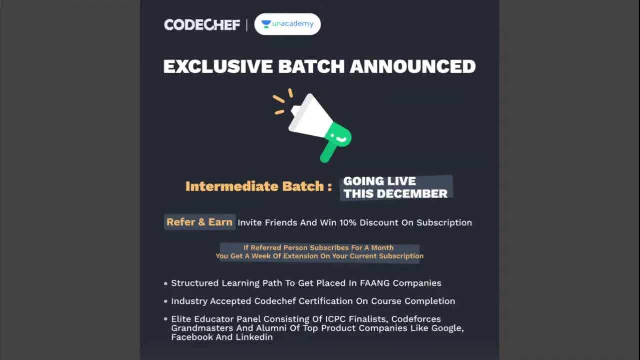 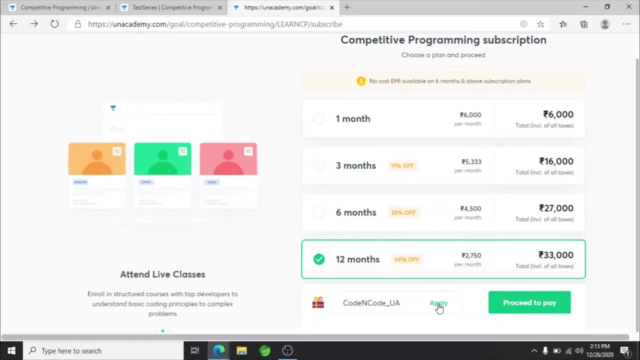 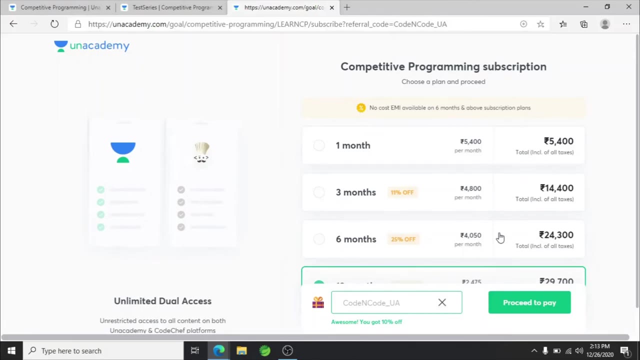 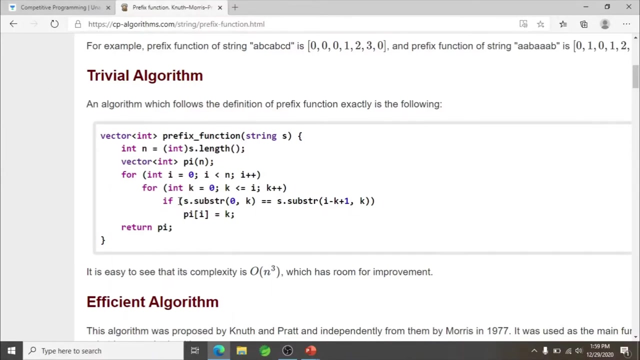 accepted codechef certification. It has just started this week, so go and join quickly. You can use my referral code and get 10% off. There you go. So let's head back to our lecture. Now that you understand the working of prefix function, now let's go back and see this code. 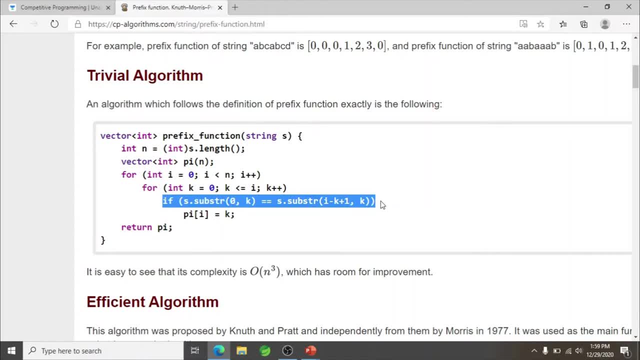 You see, this is the most expensive operation when you are comparing two substrings. When you compare two substrings, you know it requires big of n time, since we are not using hashing here. It requires big of n time if the substrings are of length n. 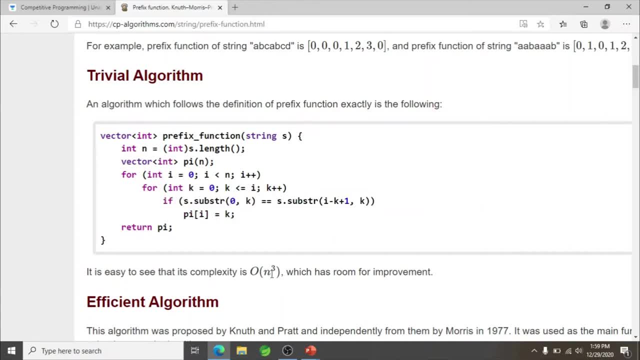 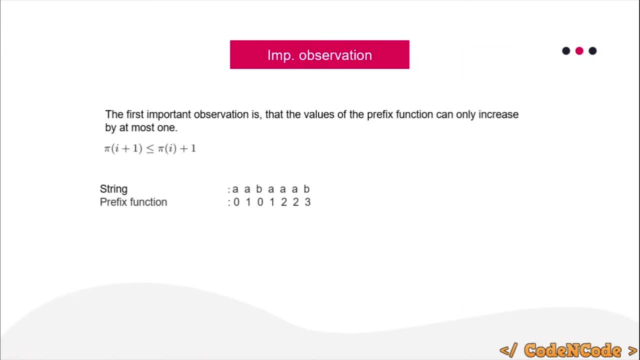 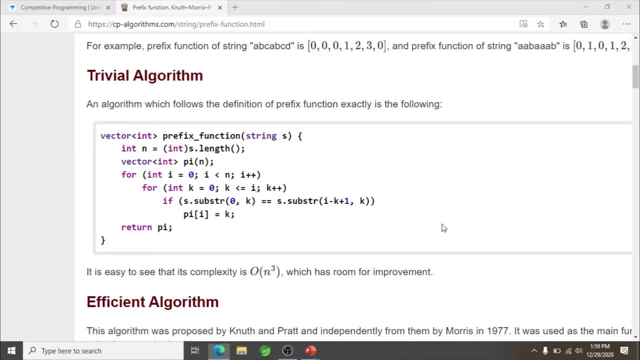 And because of this we are getting an extra n factor in the overall complexity. So the question is: can we improve this comparison? So, first thing, one of the most important observation is this: There are- we will be trying to come up with an algorithm where we do not have to compare. 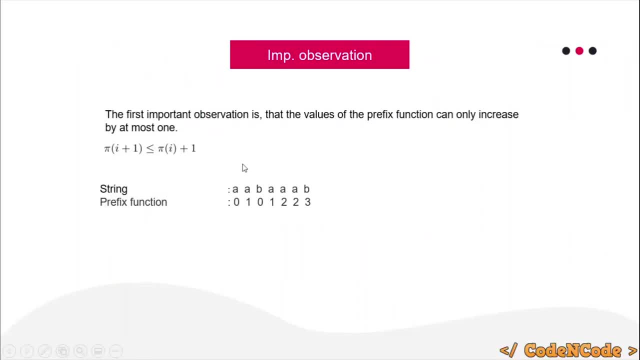 the substring. How will we do that? This is one of those important observation. There are two important observation. There are two important observation. There are two important observation or improvement that we can make. This is one of them. One of them. 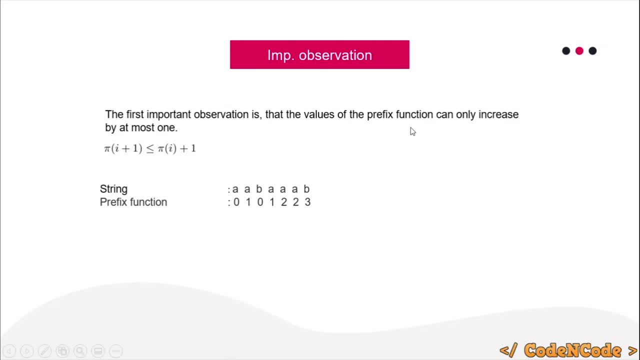 So the important thing to note here is that the prefix function can only be increased at most by one. So basically pi of i plus one would be less than equals to pi of i plus one. So basically it can increment at max by one. So here you see, it was zero, so it is incremented by one. 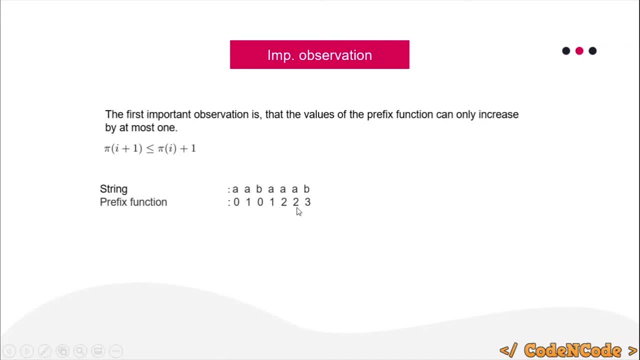 Again here. the next is incremented by one only from the previous one and this is not incremented at all. This is incremented by one only. So we can increment at most by one. It is possible that it decreases, that is possible. it can decrease by, it can decrease and go. 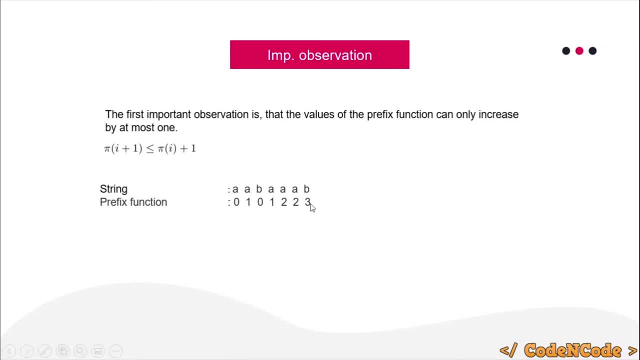 up to zero. that is possible. if I were to add x here, I guess the next pi of the next index would be zero. It is possible that it falls to zero. that is possible, but it would not increment by more than one. At max it can increment by one from the previous pi value. 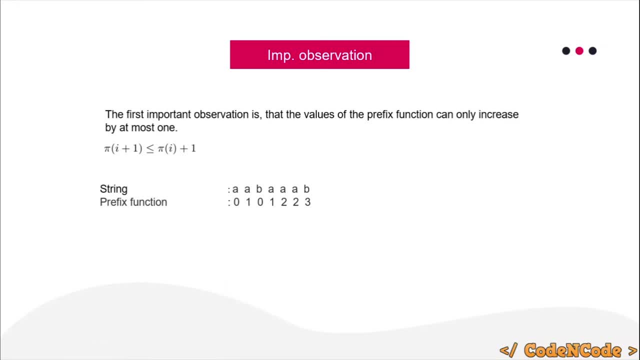 And how we are going to prove this. It is very simple to prove. You can prove it using contradiction, So I would like you to try it yourself. otherwise I am going to explain it with an example. This example you can replace with variables and make it a general case. 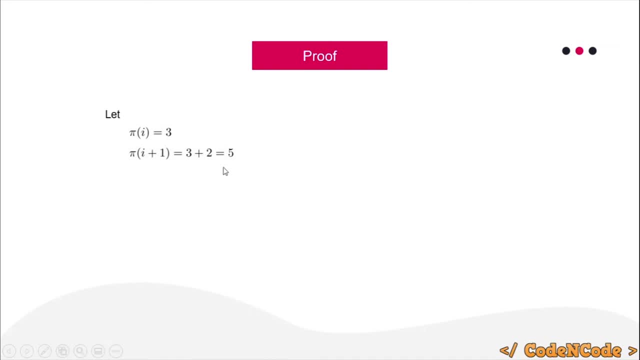 I am only taking special case so that you can understand it better. Understand it better, Understand it better. The proof remains the same. You can replace these numbers with variables and you will be able to generally prove this what I am going to show you. 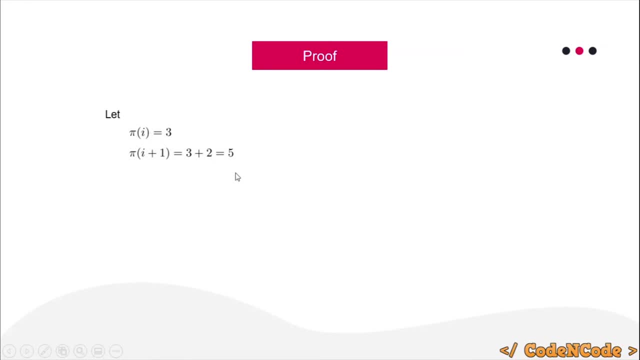 So see, suppose we are assuming. we will be proving it by contradiction, of course, because pi of I plus 1, I have taken 5, which is incremented by 2, right? So of course we are going to prove it by contradiction. So let us assume pi of I was 3 and pi of I plus 1 is equals to 5.. 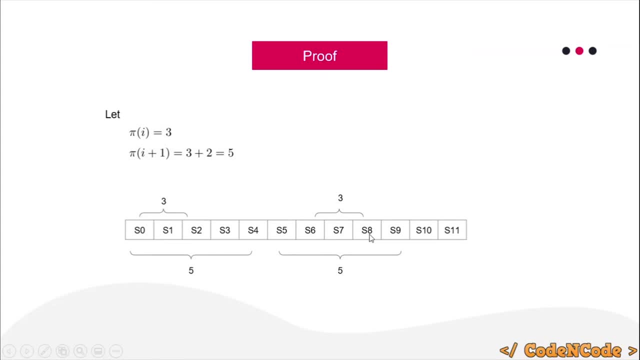 See here. Let I be 8. i be 8, so pi of i is clearly 3, because s6, s7 and s8 matches the first three characters. so basically these three characters of the suffix, suffix of length, 3 matches the prefix of length. 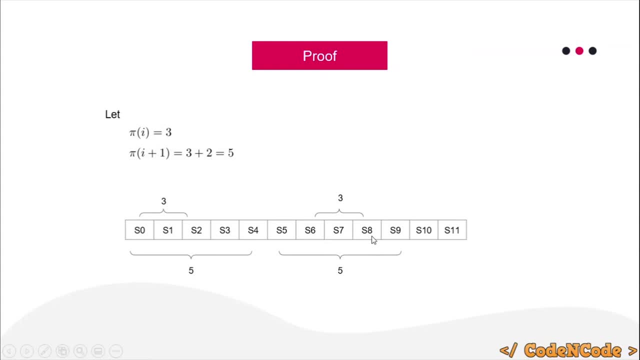 3, i'm considering i is equals to 8, right? so pi of i is equals to 3. now i'm saying that pi of i plus 1 is it is actually 5, which is being incremented by more than 1. we are saying that it cannot. 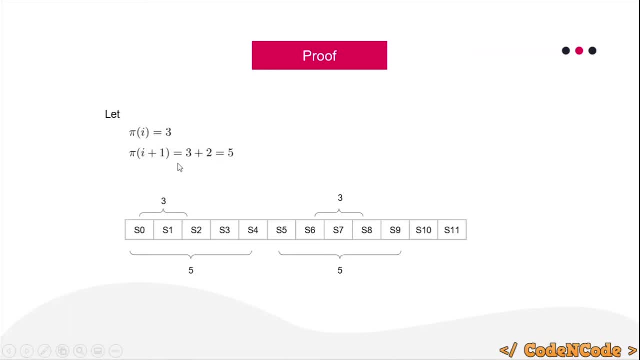 increment by more than 1. but here we are assuming like let's assume that okay, it can increment by more than 1, and so i am incrementing it by 2, or you can take any number here: 2, 3, 4, 5 or doesn't. 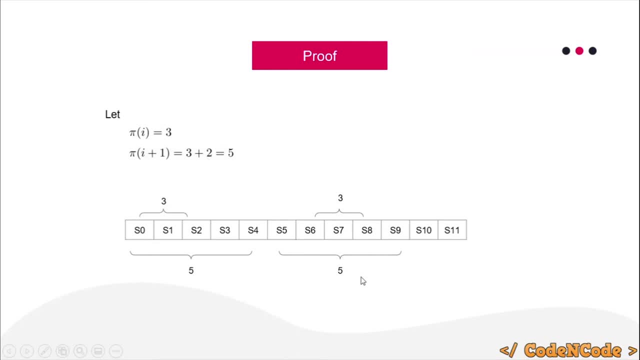 matter. so i'm assuming that i of 9 is actually 5 if that is true, so you should see here that if that is true, if pi of i plus 1 is equals to 5, that means the 5, last 5 character ending at index 9. 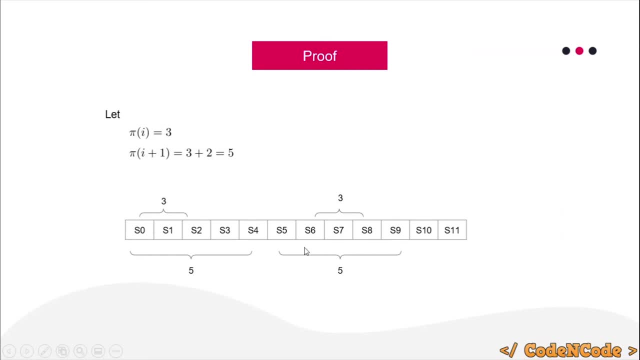 match to the first 5 character. basically, this suffix is equals to this prefix, right? what i can do is that i can take this suffix, remove the last character and this s5, s6, s7 and s8 must match right, or s0, s1, s2 and s3 right, because 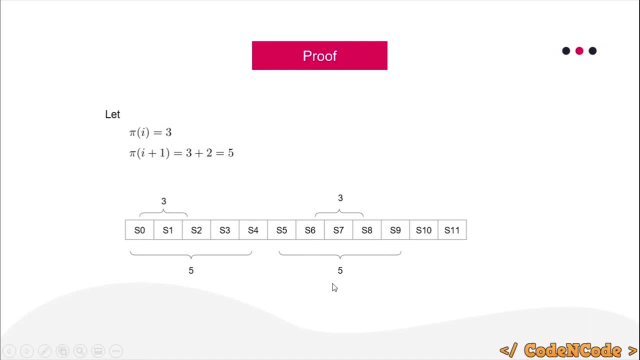 so s2, s2 and s3, right, because so. so pi of 9 is equals to 5. that means these five character may match the first five character. that means if you ignore the last character and only consider the first four character, they must match the first four character, right? if that is true, then, uh, the pi of i, which is index 8. pi of i. 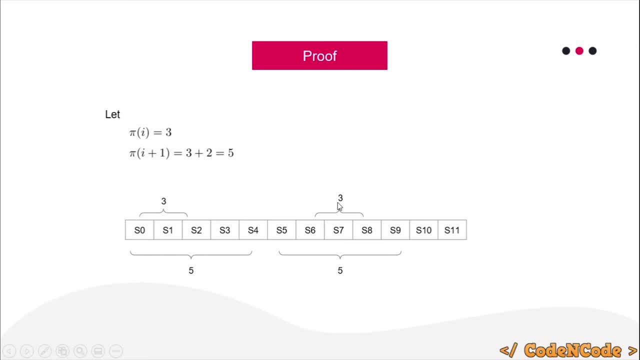 should have been 4 not 3, right? so we are uh reaching to a contradiction that pi of i is actually 3, it it shows that if pi of i plus 1- i am considering 5- then pi of i should have been 4 not 3. and then we are reaching to a contradiction that it should have been 4 not 3. 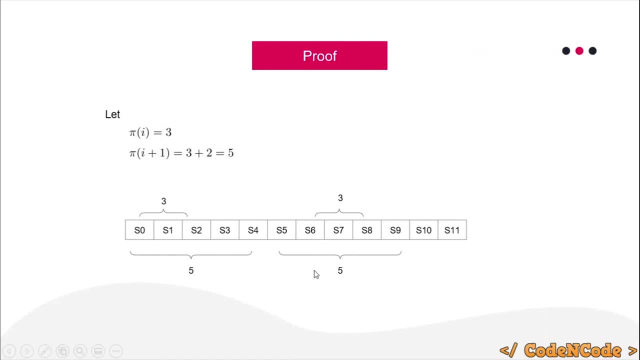 and that is why, uh, this claim is actually false and hence our original claim is actually true. so you can use variables here and using the same uh set of argument, you can prove using a contradiction. i i hope you are understanding what i am trying to say here. if you are not able to understand, just go through the uh the article. 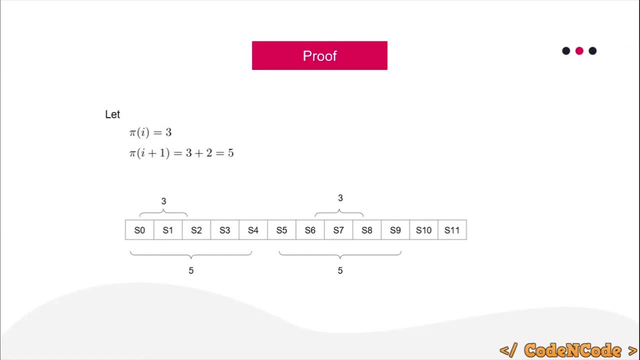 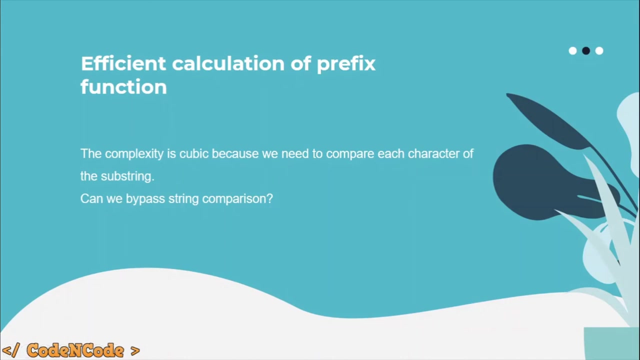 there on the cpalgorithmcom, the link which i'll be providing, there's a description. if you are not able to understand, even though, please mention it in the comment section, i'll be trying to help. so this way you can prove. so now we know that perfect function increments at max by 1 right. 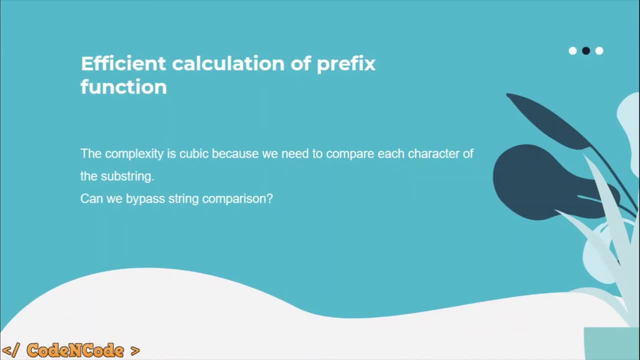 now, uh, how is that going to help us light an algorithm which is efficient enough? so let's see how. so the clearly this- i have already mentioned the cubic algorithm or the cubic complexity- is because of we are comparing each character, because when you are comparing two substrings, 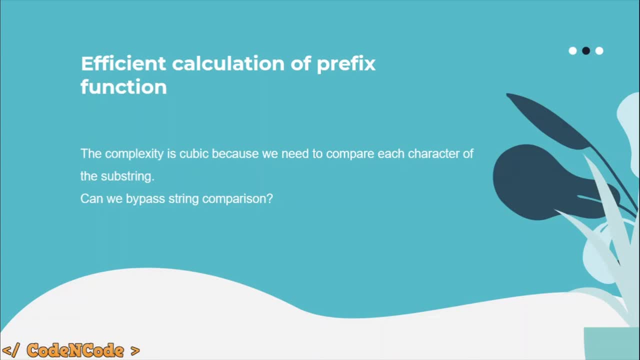 they are actually being compared internally by their characters, right? so can we bypass the string comparison? now we are going to answer this question. so see here: if we compare the numbers, they are actually being compared internally by their characters, right? so can we bypass the string comparison? now we are going to answer this question. so see here, uh. 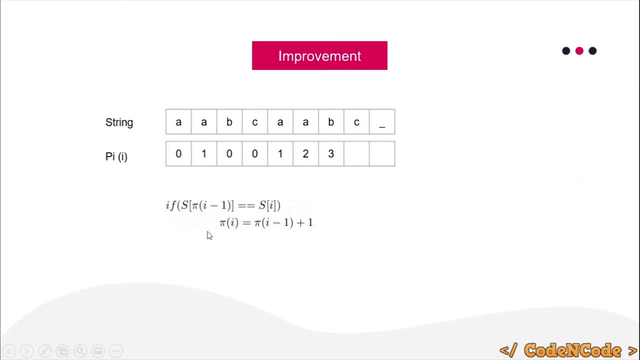 we are going to get junior Hail covid and disqualify the Prison Constitution now and we get this faculty healthy. madam California Understudy Tamara Flood, joining class 5 undergrad student. So see here, this is an important, this is another improvement and this is an important. 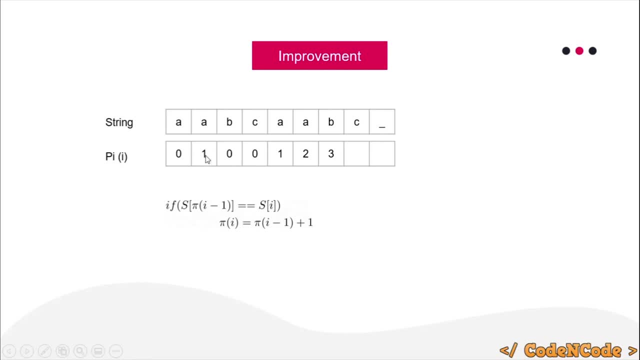 condition. See here, suppose from 0 to i minus 1, I am considering this index to be i minus 1, I have already calculated right Pi function from 0 to i minus 1, I have already calculated. Now I am going to calculate pi of i. To calculate pi of i, I need to do this, I mean. 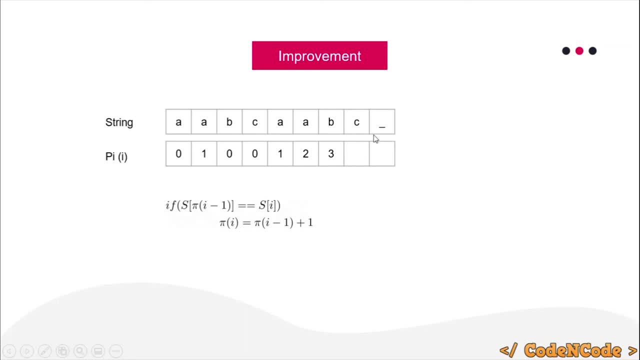 what I have to do. we already know that pi of i minus 1 is 3, so pi of i can be at max 4, right? So if pi of i is actually at max 4, that means these 4 characters must match. Should I compare? 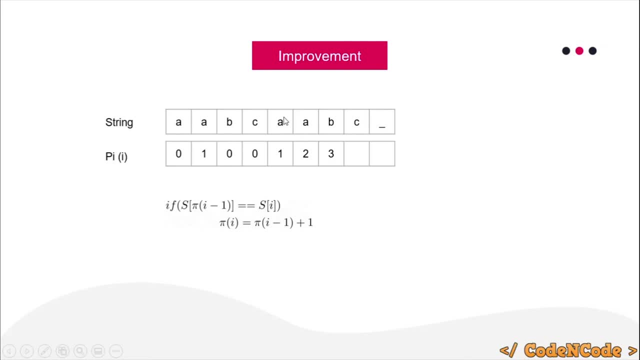 all of these 4 characters, with these 4 characters, to see whether the pi of i is going to be 4?? The answer is no. I don't have to. Why? Because pi of i minus 1 is 3, that means the first 3. 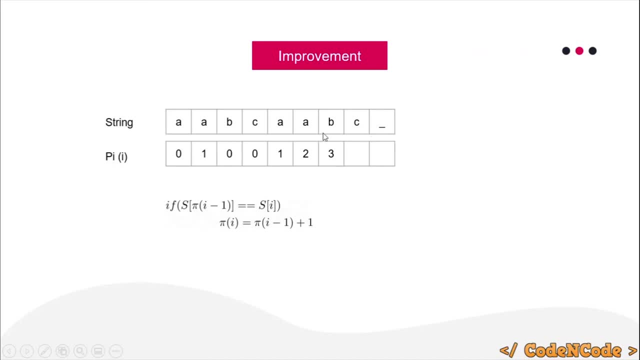 characters already are matching. So I don't have to compare the first 3 characters, I only have to compare the fourth character. So there is only one comparison. There are not. all of the characters are not being compared one by one. only the last character is being compared. So pi of i minus 1 is 3,. 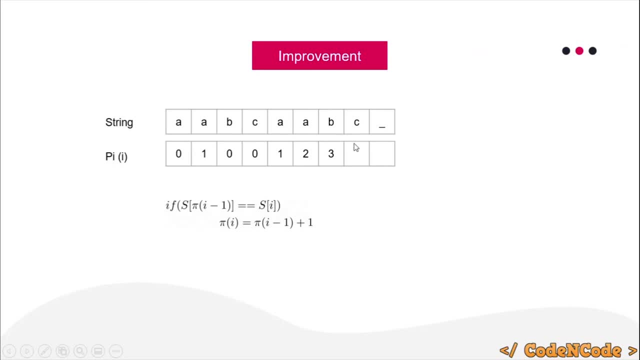 that means first 3 characters are already matching. If pi of i had to be 4, then the fourth character must match the fourth character or prefix right. Fourth character's prefix is at position Pi of i minus 1, right. So that is why I am comparing the fourth character, which is pi of i minus.